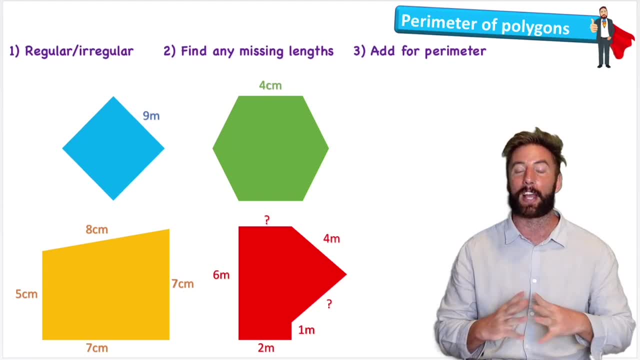 What is up everybody? Welcome back to the Maths Guy. Today we are going to be looking at how to find the perimeter of polygons. Let's go Okay, so we have these range of polygons here on the screen. It's probably an important time to just mention what a polygon is. 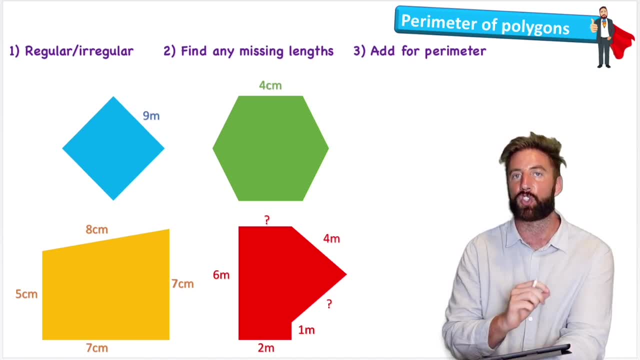 So a polygon is any 2D shape that has straight edges and is a closed shape, which means that our sides join together. We also have two types of polygons. We have regular polygons and irregular polygons. Our regular polygons are those that have the same size, length and the same angles. 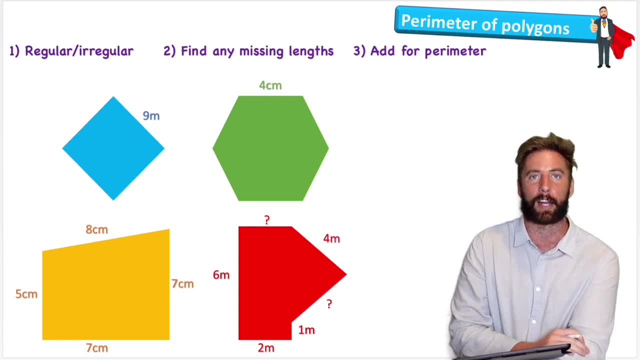 And our irregular are the ones that look strange, with different lengths and different angles. So what are our steps to finding the perimeter of these polygons? Well, the first step is to identify if it's regular or irregular. Then we're going to find any missing lengths. 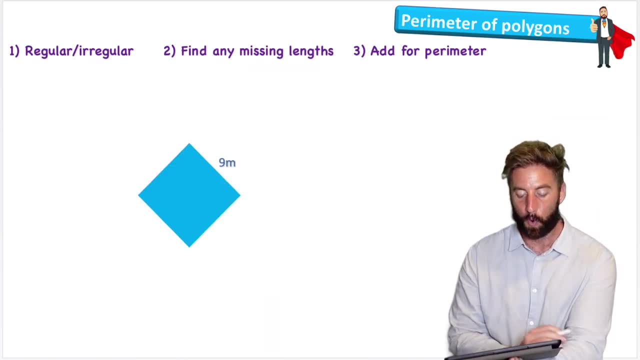 And then we're going to add to get the perimeter. So let's look at questions. Question 1, we have this square Now the first job was to find out whether it's regular or irregular. Now, in this case, our shape is regular because it's a square. 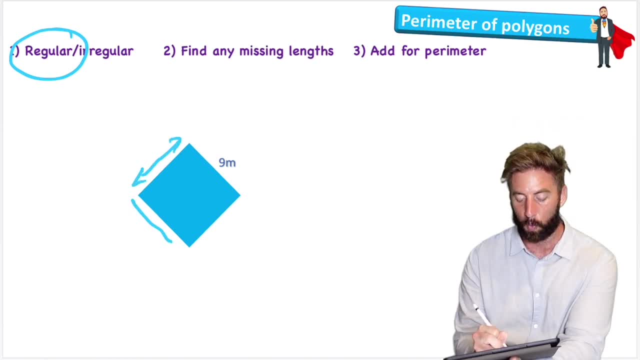 And a square has the same length sides all the way around. So therefore, when we get to our find any missing lengths stage, we know that if one side is 9 metres, then all sides must be 9 metres. So then we just add for the perimeter. 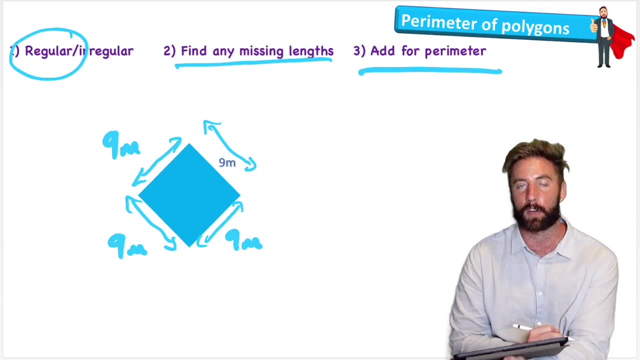 And all that means is we're going to add, We're going to add these measurements around the outside of our shape to learn the perimeter: 9, 9,, 9 and 9 is 36.. Now what you might have noticed is that we're just adding 4 sets of 9 to each other. 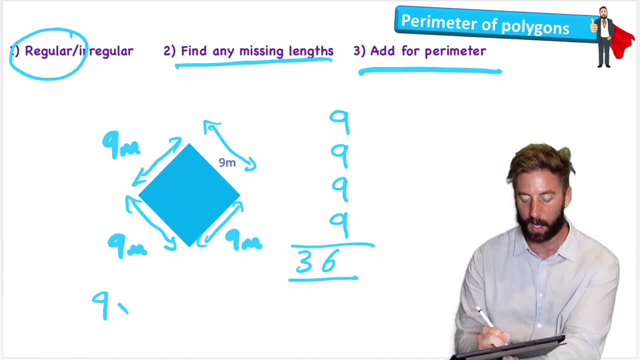 So we actually have a simpler way, don't we? We could do 9 times 4, because there are 4 lengths. 9 times 4 is also 36. And therefore, using this knowledge, with a regular polygon, we can actually make a formula. 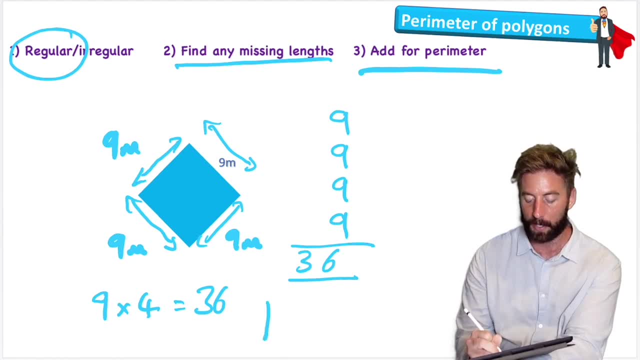 And we can say that our formula here is perimeter. And we can say that our formula here is perimeter, which is our actions. next figure on bar: follow me. This is our function for 0.. And the 8 games for 2, we'll be adding 4 sets of 9enti. 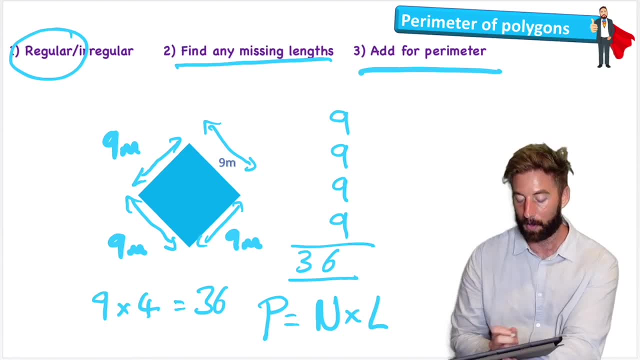 1, 6,, 7,, 8,, 6 and 10 times 4.. 1, 6, 5, 6 is 6. Then w is going to be more than 4 and we'll have 3 sets. 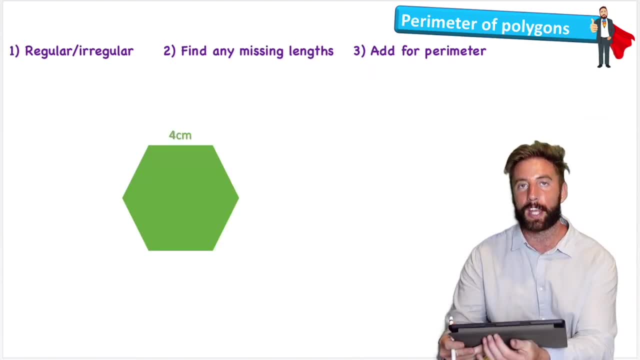 5 times 4 is 2, and that somehow�CIA 5 times 4 is 12 units. 5 times 6 is 0.. 5 times 4 is 7m, And the result will be the least we can have is the euroでは. 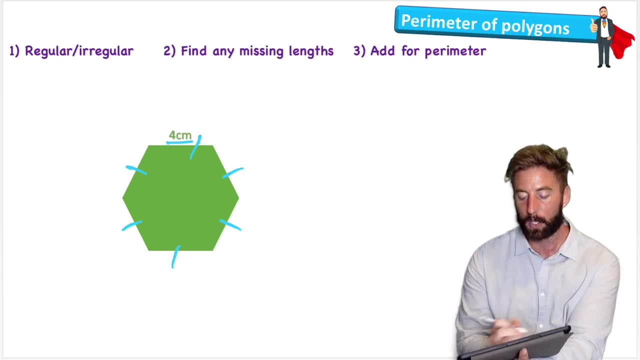 So you might qualify 17 for losing one turn. The worst problem is that we don't have a real pockets left. Let's continue formula in place. this time I'm going to say p equals number of lengths times the length itself. so let's now put our numbers in. we have p equals. well, how? 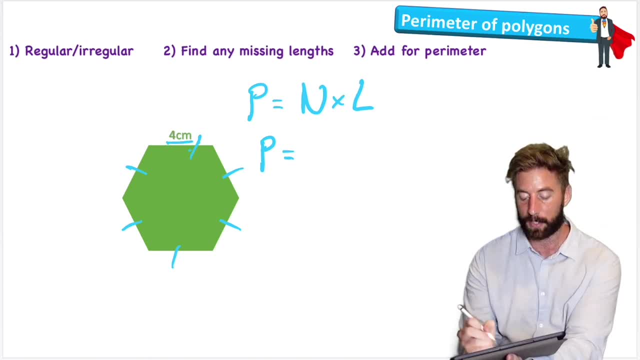 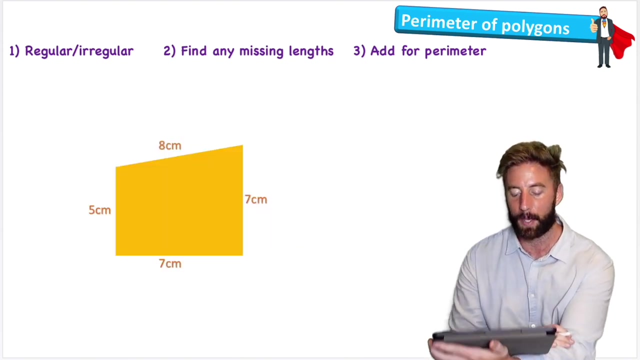 many numbers of lengths do we have? we have one, two, three, four, five, six, like every hexagon. what was the length? four, so p equals six times four. therefore p perimeter equals 24. pretty easy for a regular polygon. let's see what happens now with an irregular polygon. let's have a look at this shape now we can clearly 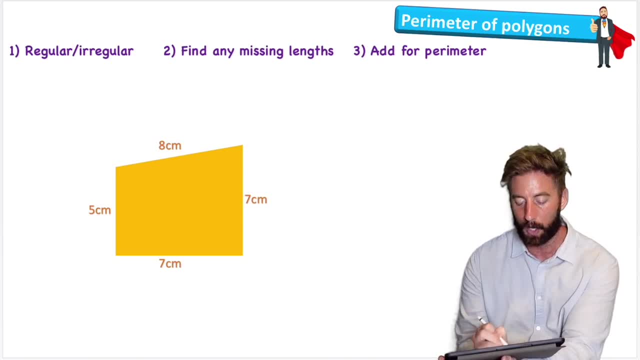 see that this is an irregular polygon straight away because, look, we have different size, lengths and even without those numbers, we can probably see that that is a regular, because we have lengths over here longer than this length here, for example. we also have an acute angle, here an obtuse angle and two right angles, so all our angles are different. 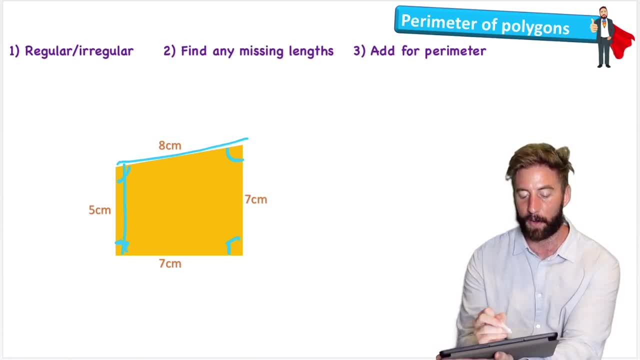 as well. so this is not regular at all. this is very irregular. so can we use our formula? well, no, because we did p, times number of sides, times the length. well, which length? there's lots of different lengths. so, unfortunately, irregular means we cannot use a formula. we have to go back to the 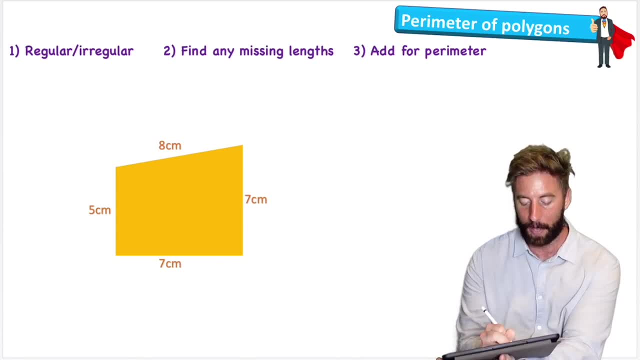 old-fashioned method of adding up our size, so we have a properly well defined cross rectangle here and something we could simply do now. in that case, 5 and 8, a 7 and a 7 centimetres, 5 plus 8 is 13,. 13 plus 7 is 20,, 20 plus 7 is 27.. 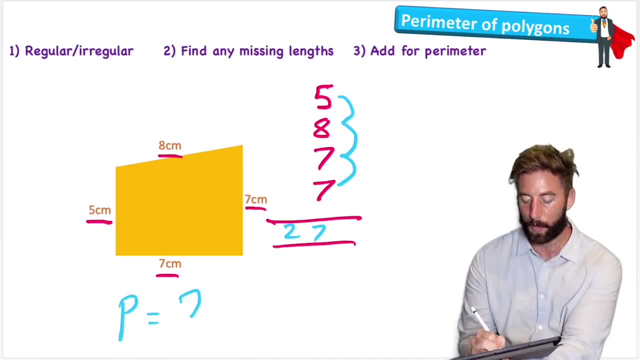 So for this one, my perimeter equals 27 centimetres, So it's pretty straightforward, even if it's irregular, but only if we're given all of the lengths, Because we could clearly see here this length was 8 centimetres, then we had 7 centimetres, another 7 and 5.. 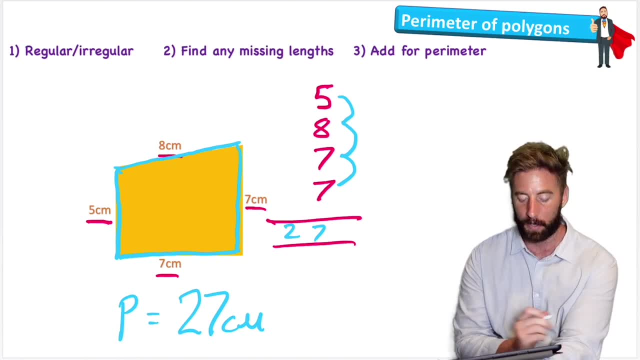 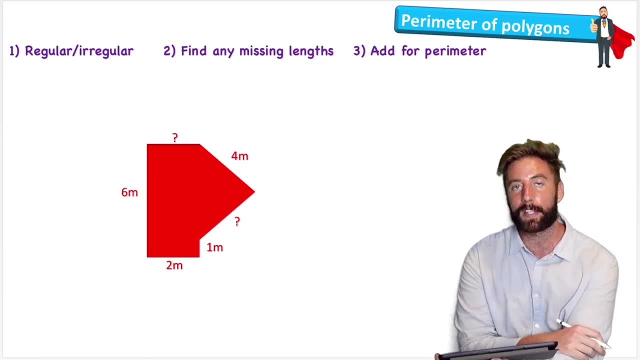 So we could create all of our perimeter with the numbers given. What happens if we have some missing numbers? Well, here we go. this is another example, And what we have to do in this situation is we can't just add the numbers that we're given. 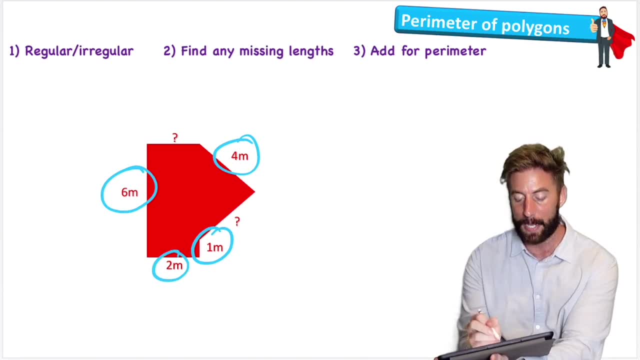 because we'd end up missing lengths- We would miss this length here and we would miss this length here- And obviously that would not be an accurate perimeter, therefore. So we have some work to do, We have to look at the information we've been given. 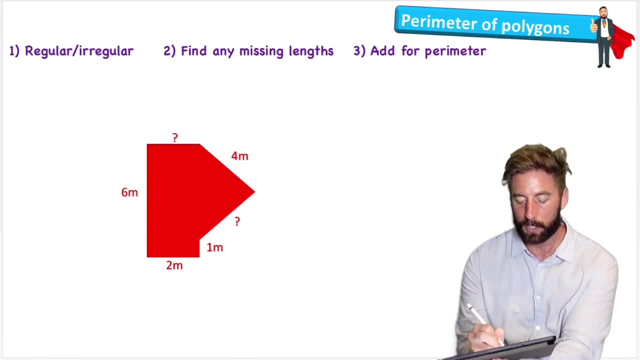 and see if there's any clues to help us. So let's look at this one first of all. I'm looking for that question mark. Well, I think I can look opposite and see that this is 2 centimetres, And if this is 2 centimetres, then this will be 2 centimetres too. 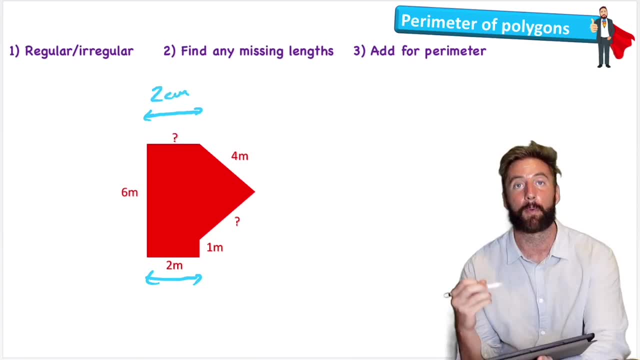 So let's label that 2 centimetres. But again, I'm still not done, because I have this missing length here And this missing length might be a little bit harder to spot, but if we look on the opposite side again, I can see that we have a length being given to us of 4 centimetres. 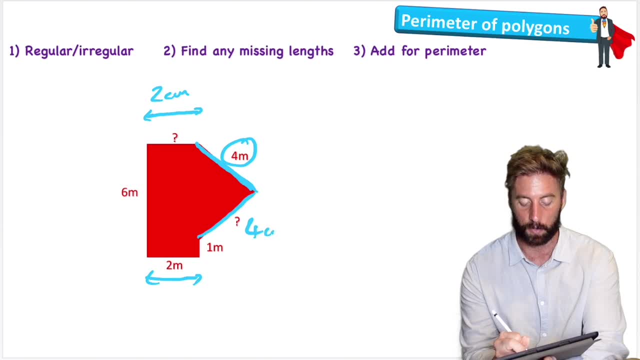 and therefore this must be 4 centimetres too. OK, now I have all my lengths. We can check that by going around our perimeter of our shape and make sure we're not missing any lengths. Now I can add it up. 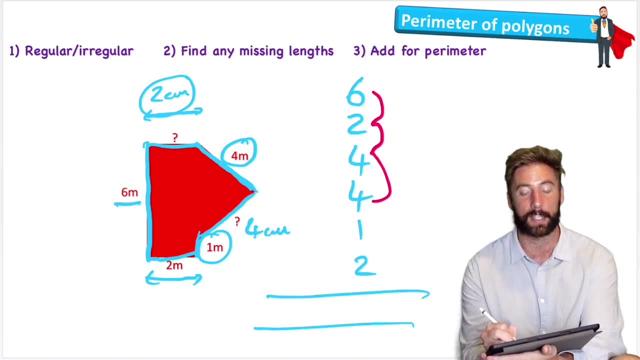 6 plus 2 is 8,, plus 4 is 12,, plus 4 is 16,, plus 1 is 17,, plus 2 is 19. So perimeter equals 19. Metres. Don't forget to put your measurements. 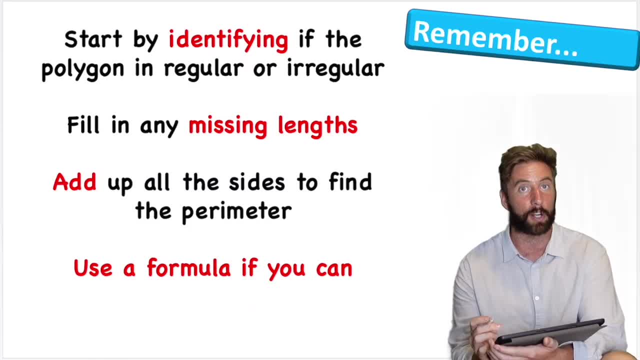 OK, and there we go. That is, finding the perimeter of a polygon. So let's look at what to remember. Start by identifying if your polygon is regular or irregular. Fill in any of the missing lengths and add up all the sides to find the perimeter. 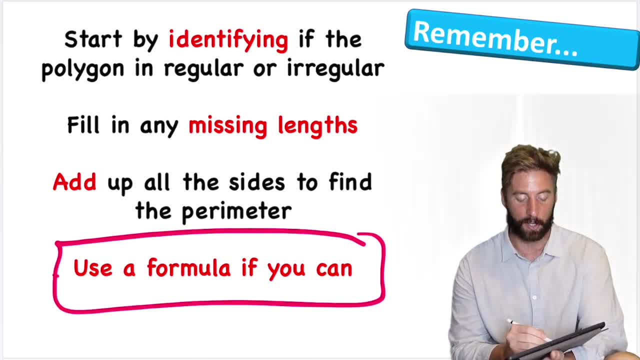 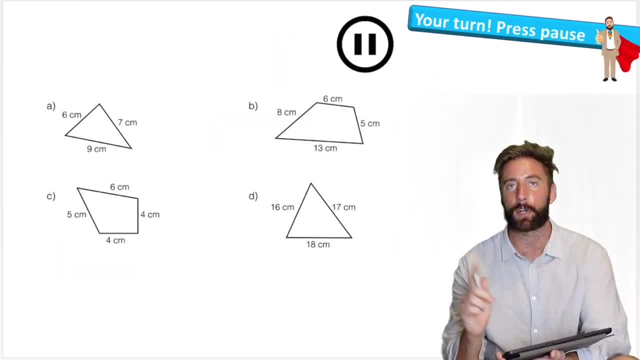 Use a formula, if you can Remember that our shapes have to be regular to do that. OK, here are four questions for you to have a go at. Put your answers in the comments section. press pause on the video now and take your time. 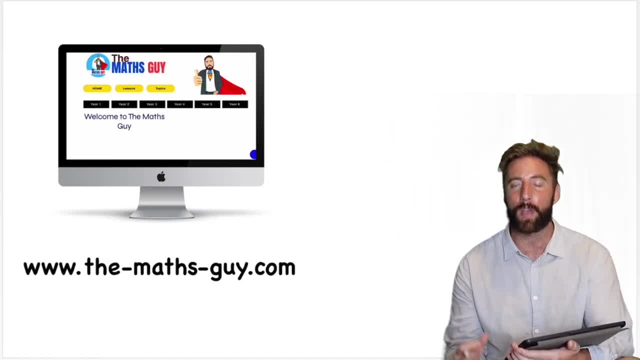 And there we have it. Hopefully this video was helpful for you. If it was, think about subscribing to the channel or check me out on my website, But for now, peace out.